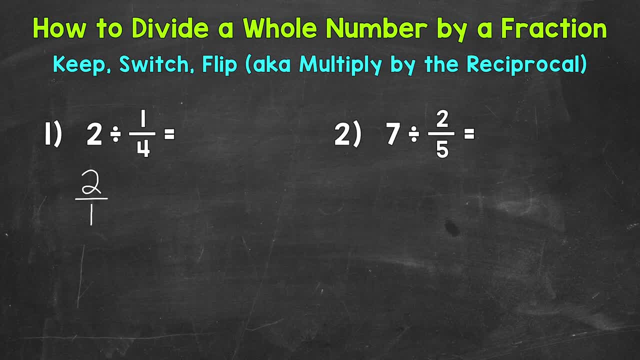 Whenever you rewrite a whole number and put it in fractional form, all you need to do is put it over one. Now the the purpose of this. we want to have a numerator and a denominator, So we kept the value of two there. 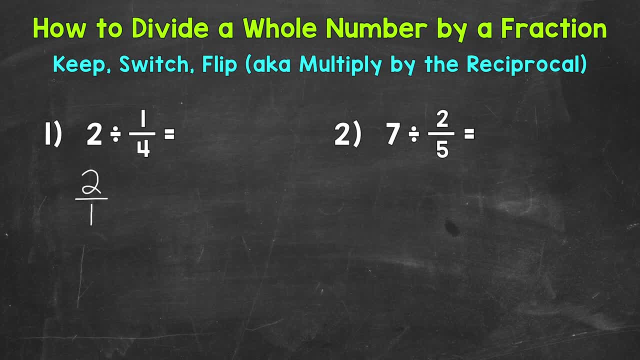 We just put it in fractional form. Then we switch from division to multiplication And since we switched to the inverse or opposite of division, we're going to need to flip the second number or fraction In the case of number one, here we have a fraction. 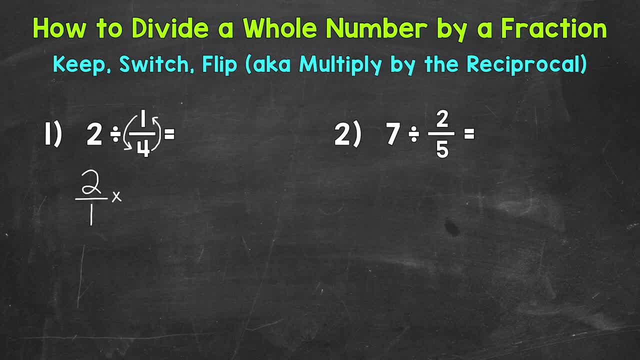 So the denominator is now going to be the, the numerator, And the numerator is now going to be the denominator, So we have four over one. Once we get to this point, we have a multiplying fractions problem, which we just multiply straight across. when we multiply fractions, 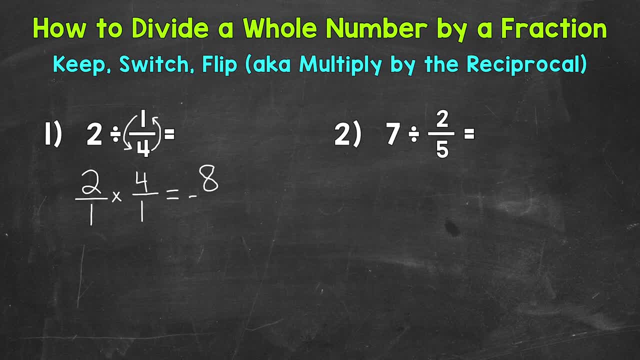 So two times four is eight and one times one is one. So we get to the answer of eight over one, which is an improper fraction. So we do not want to leave it like that. This is going to be eight. Our final answer is eight. 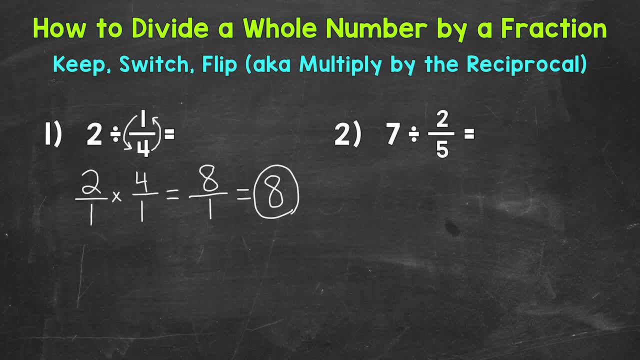 Two divided by one fourth equals eight. Let's move on to number two, where we have seven divided by two fifths. So we are finding out how many two fifths are in seven, so to speak. So keep switch flip. 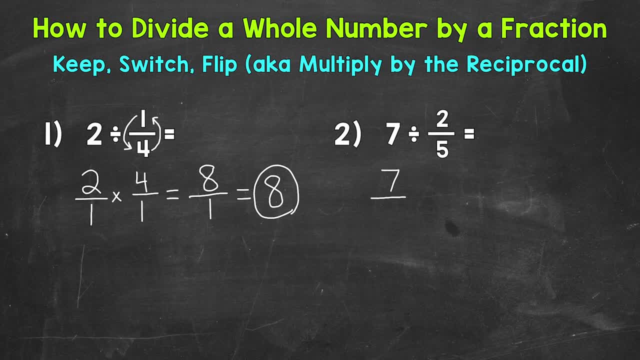 We will keep our seven, but put it in fractional form by putting it over one Switch to multiplication and then flip our second number or fraction. Now we can multiply straight across. Seven times five is thirty-five, and one times two equals two, So our answer is thirty-five over two. 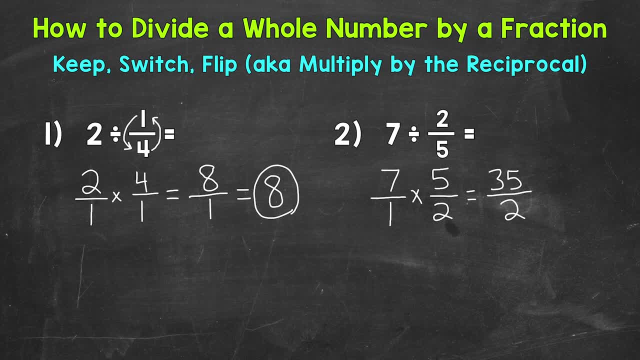 Now we don't want to leave it improper. We want to convert this to a mixed number. So we do Five divided by two. How many whole groups of two are in thirty-five? Well, seventeen. So that's our whole number of our mixed number.